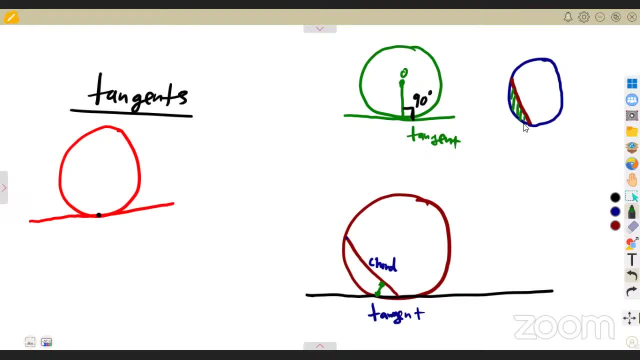 There is this region here. What is it? this one? But that was our introduction, This one on our introduction, Let's go back to our intro. We said we talked about this. We said that that region it is a special, it is a name. 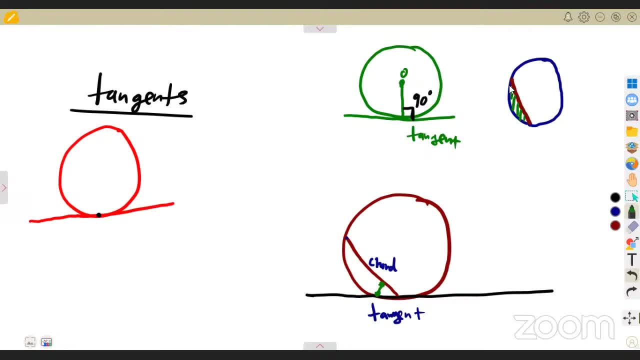 There is a code, this one, and this, this line, It's a code. Then there is this part here, the region of an arc, This one, I want the part that is shaded, this one inside this one. It's what a segment. But what it does now is: 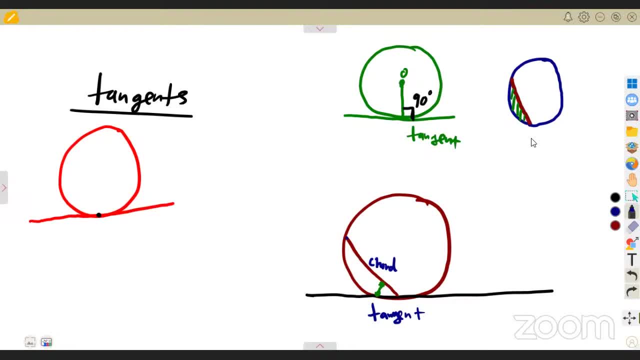 that if you check there too, because our code is from the code. Let's go back to this segue. Let's say it is passing through the what, through the center. If it passes through the center, the only special thing is that it passed through the center, so it's. 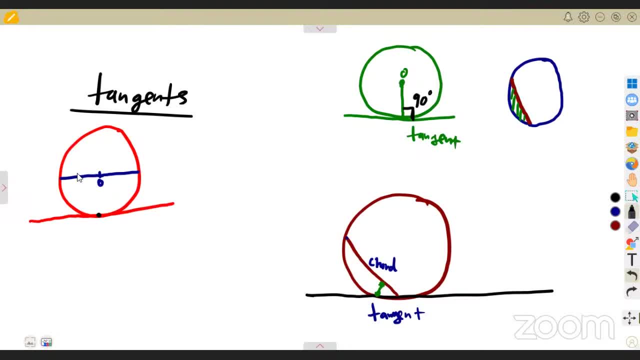 now called a diameter, But it's a code, Still a code, And it was creating two regions here: this region and also another region, this side, a segment. But these two segments are equal in size, so they are special segments, semicircle. 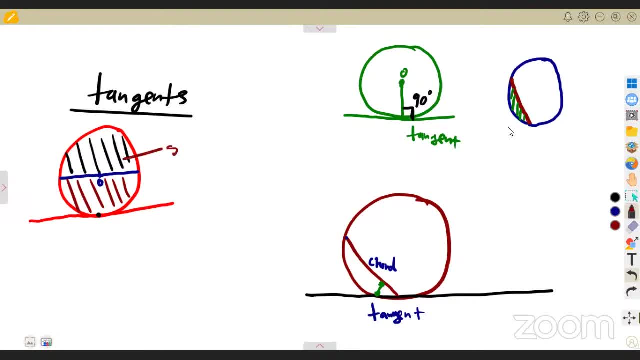 We are now talking of what. That is the only part to say. a diameter is just a special code And this region here, which is our, our, our segment, is just a special segment. to say now, it's referred as a what, as a semicircle. So 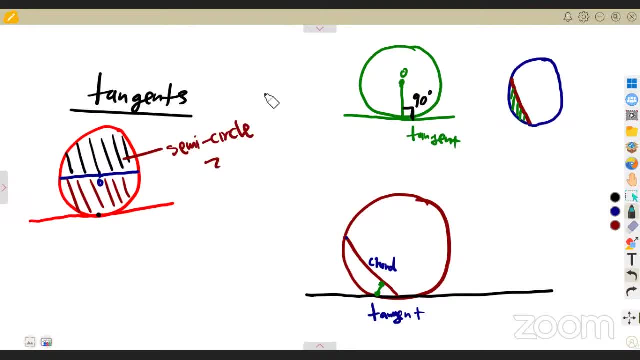 with, without this knowledge or without this idea of this segment. it means this theorem is going to be difficult for us to understand. So, meaning to say, a code, when it is drawn, it is giving us what? two regions, two segments. So there's this one And there's also this one. 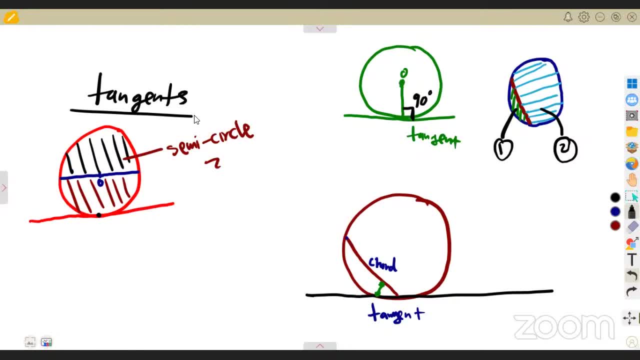 I don't know if we're together there. So I want us to understand, because this is the part of our theory, that is the part of our theorem here, This code that we just run here, this code, it is now separating our circle into two segments, two regions: this region and, this time, second. 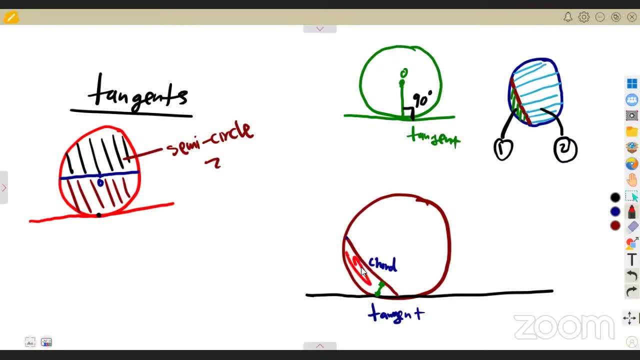 This is a part of anything here. don't talk about being one voice here. This is just a feather. This is a- soil and this region. so the theorem is: the angle between this tangent and the chord is equal to the angle in the alternate segment, which is opposite. alternate means opposite, so the word now. 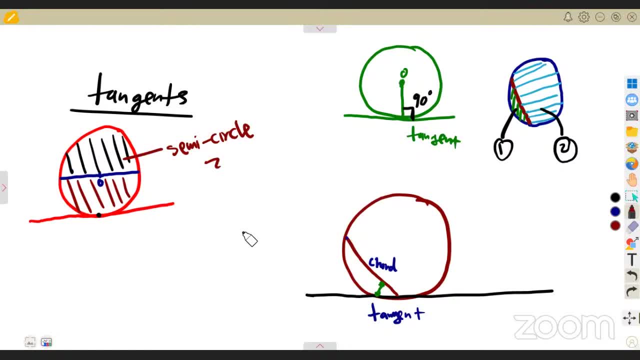 segment is there, but they're saying opposite. okay, so it's like this. so that is why i was mentioning about the issue of what? the issue of the segment, because this chord here, this is our chord, it between the tangent and the chord, this is the angle that we have. 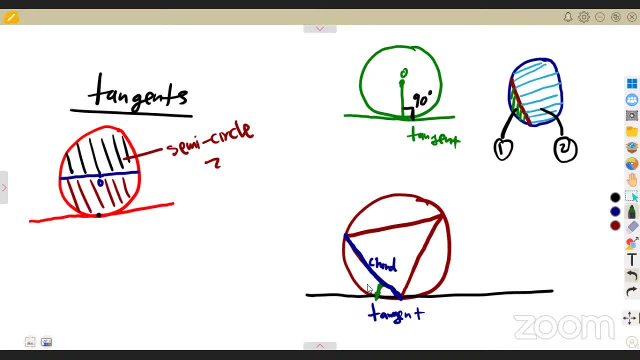 where is this angle? are you seeing that this angle is on this side of the segment. this side, so now the the, the theorem is the angle that is we are seeing here- is going to be equal to the angle in the opposite alternate segment, meaning to say, the opposite segment. it's this side here. this is where. 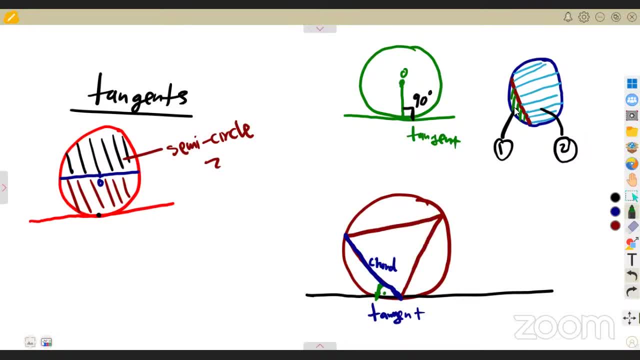 our segment, the other segment, like we saw this segment and other segment. so in this segment, where is the angle created by this chord? this one, the chord is creating the angle where, let's say, we've got points uh, a, a, a, a, b and c. where is this chord creating an angle in that segment? 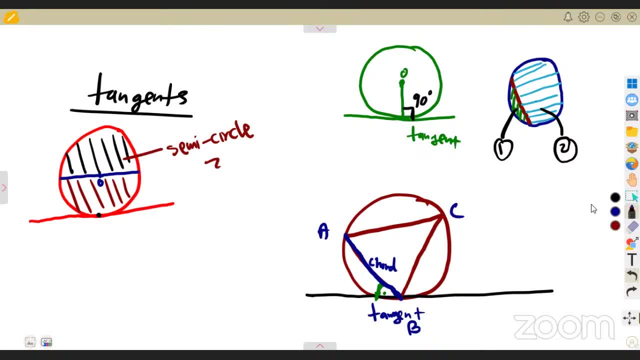 hello, this chord a, b. where is it creating the angle? what let's see to create, to subtend? where is this chord subtending the angle? where is it subtending b and c? where is this chord creating an angle in that segment? it subtends the angle here. it creates the angle at c. so it follows that this angle and this angle are. 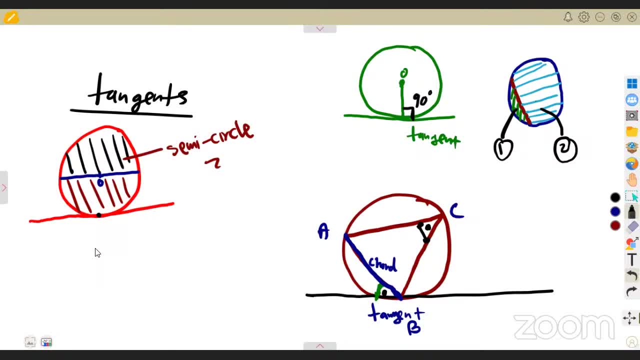 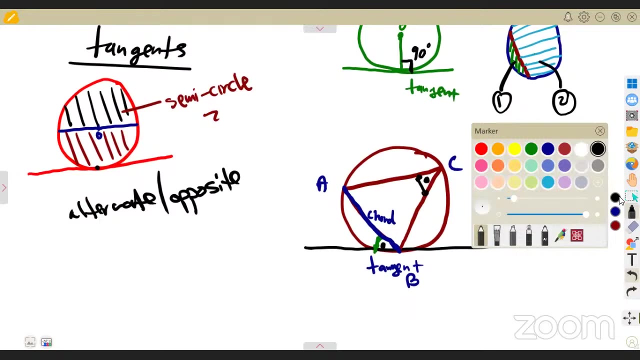 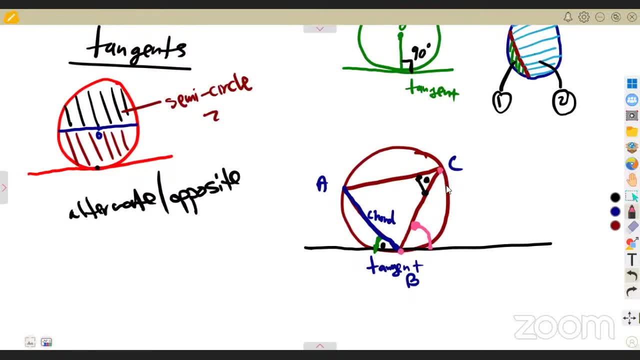 If you hold this point and this point, where is the angle going to be created? A At A exactly. So this one At A Where the angle is created, that is where we are referring to. So this angle at A and this angle between here will be equal. 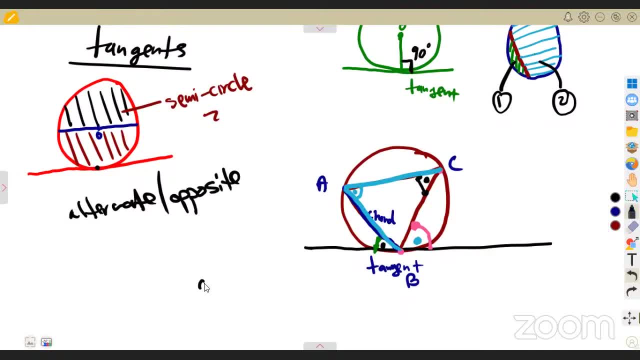 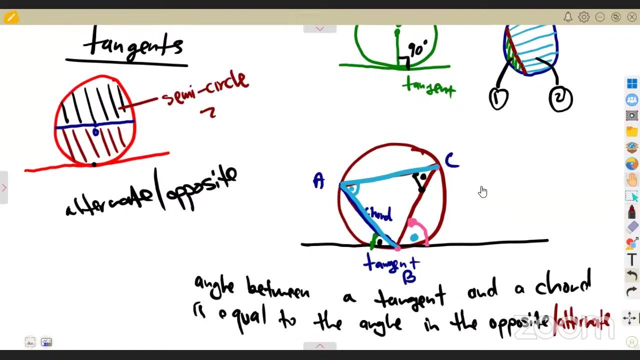 That is our theorem. So angle between a tangent and a chord And a chord is equal to the angle in the opposite segment. So The opposite, there is simply alternate. So are we seeing the idea there of the segment where it is playing a role? 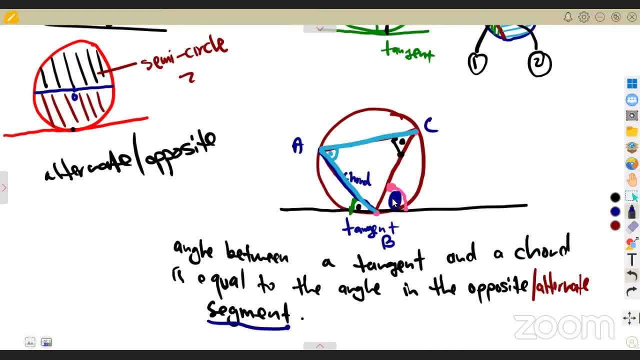 This part, The angle that we are given. it's in this segment, So the one created must be in the opposite. So where is the chord between this chord? Where is this chord creating the angle? It is creating the angle At this point. 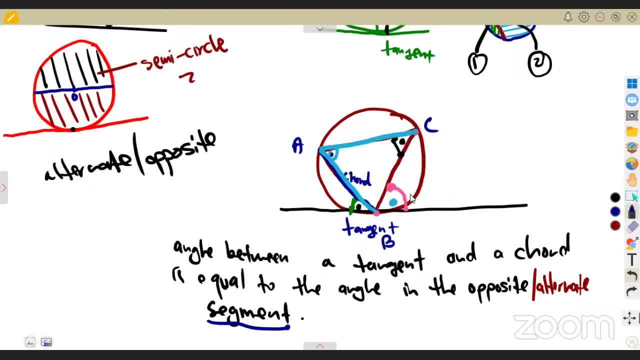 Where it is creating the angle, that angle is equal to. So if this is X, it also means this angle will be X. If this angle is Y, here it also this angle is going to be what It's going to be: Y. 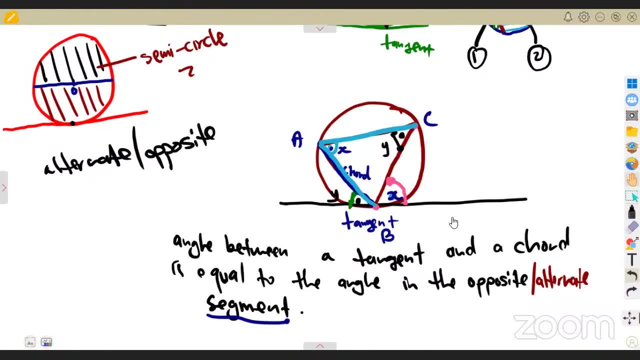 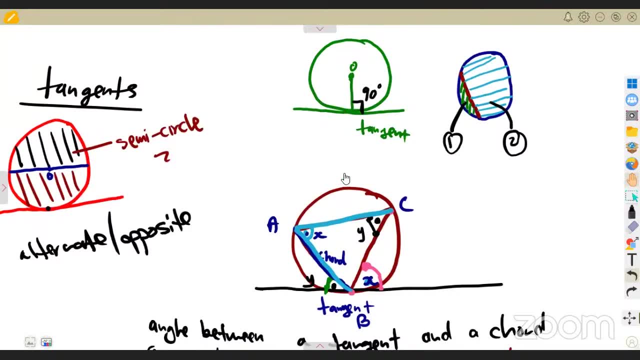 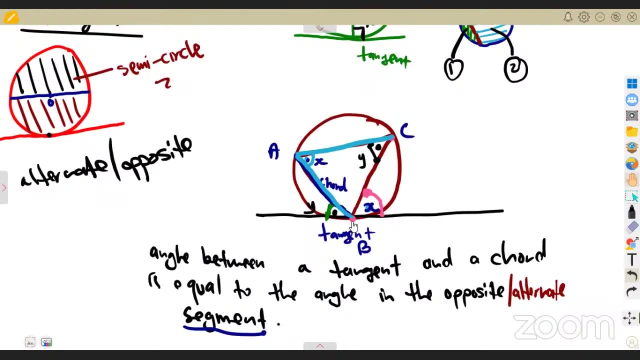 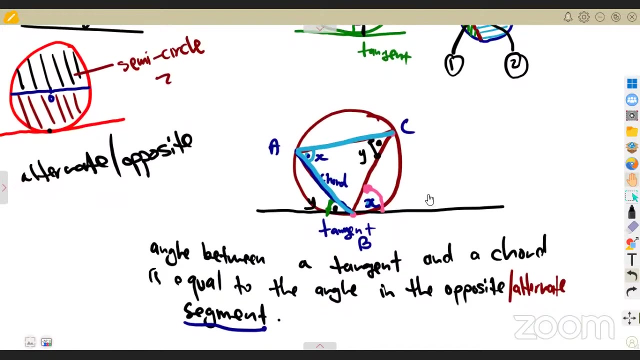 So this is the part of what A tangent. So we have this part A tangent and a radius at 90 degrees. Now we have got this part of a tangent and a chord. All right, The same tangent that we are, the same tangent that we are seeing here. they can be drawn like this: 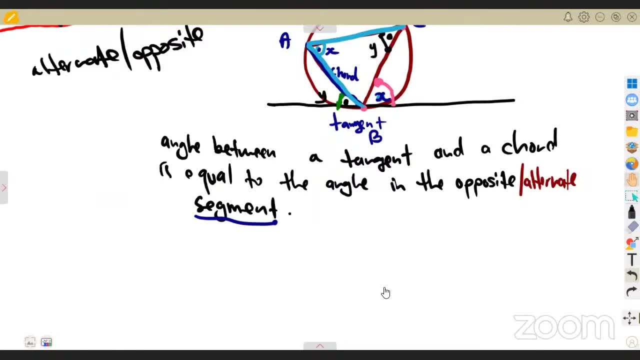 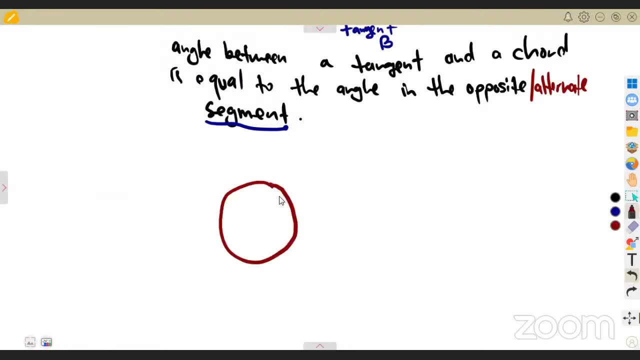 The same tangent that we are seeing. it can be drawn in this manner, We can have it from a circle in this manner. So meaning to say, when it is given as two tangents, Now we have to consider, to say that's another part. now. 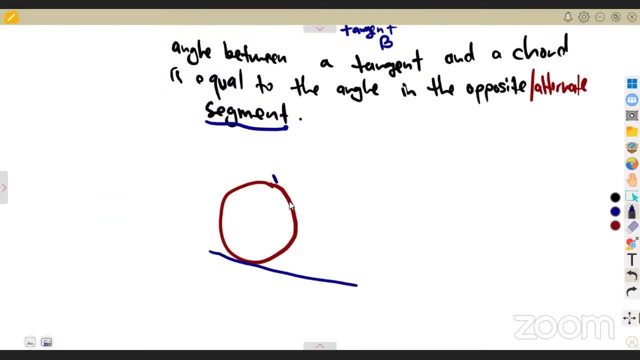 They can be two tangents like this. So this theorem, I'm going to extend it so that we understand much from what we had before. So it follows that when two tangents are drawn from the common point or from the same point, Let's say: 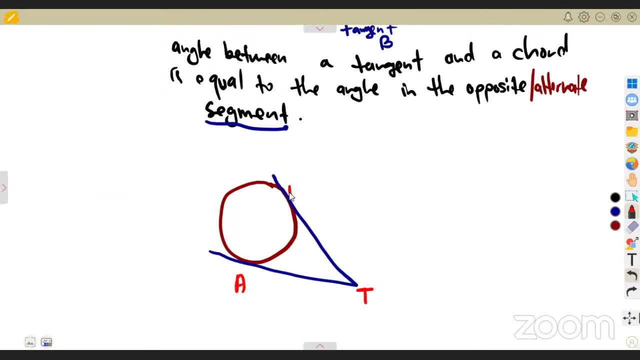 they are drawn from the point team. This is a, this is B, BT is a tangent, 80 is a tangent. These two tangents, they are equal in length, So it follows that, two tangents. So let let me just write this one so that I conclude everything. 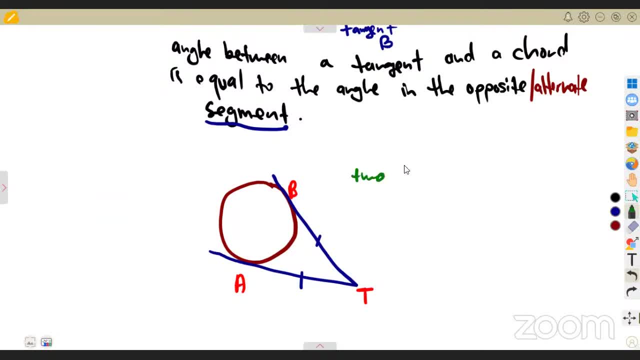 So we are saying two tangents From two tangents drawn from the same point- sorry for that- drawn from the same point to the point of contact, to the point of contact with the circle, are equal, Not equal. Okay, Okay, Okay. 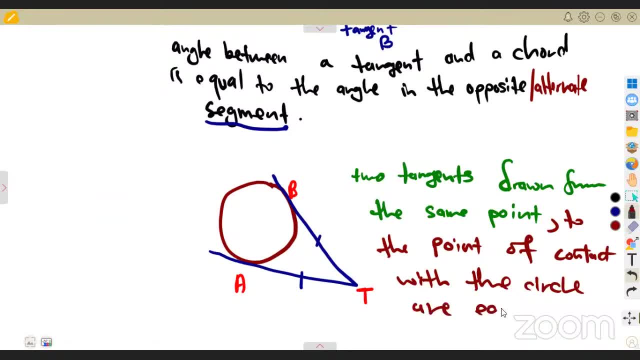 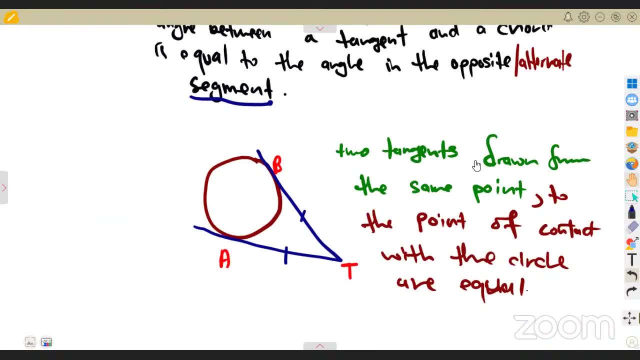 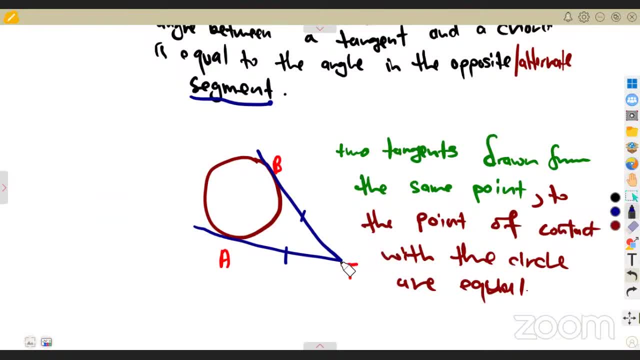 The point that we are referring. there is point t, point t, So this is a certain contact point. so definitely from this, this is our tangent, our tangent here we are referring from point B, from B, so from B to T, it must be equal. from what? from A to 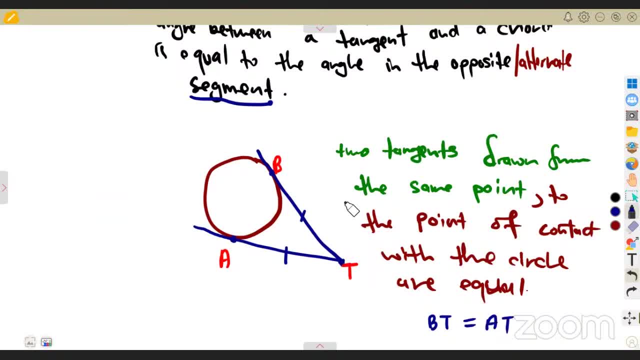 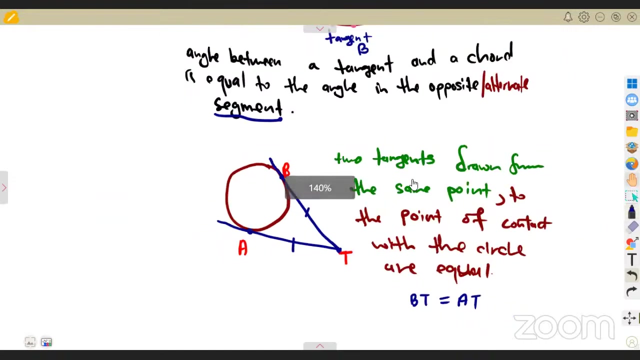 to T. that is the idea there. I don't know if we are together. are we together? yes, okay, all right, no problem. so when we are referring to a tangent, we are done when we are referring to tangents, and we are actually done. but this is it now. 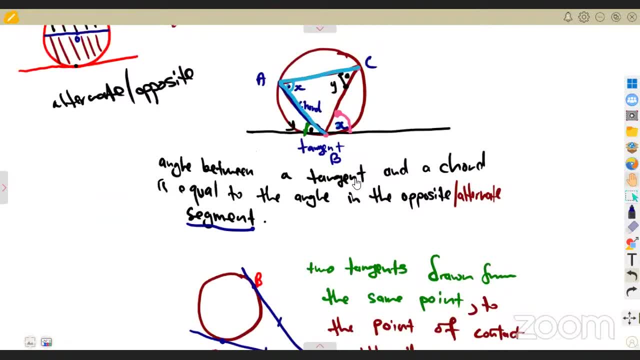 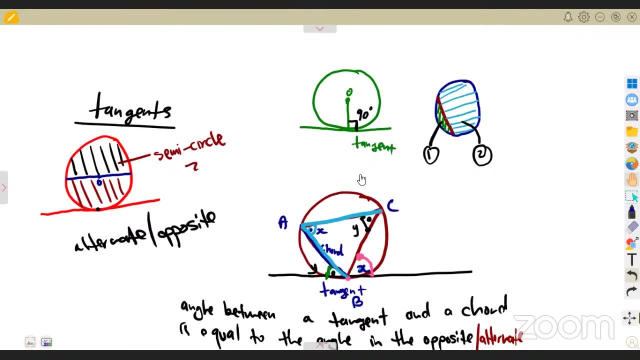 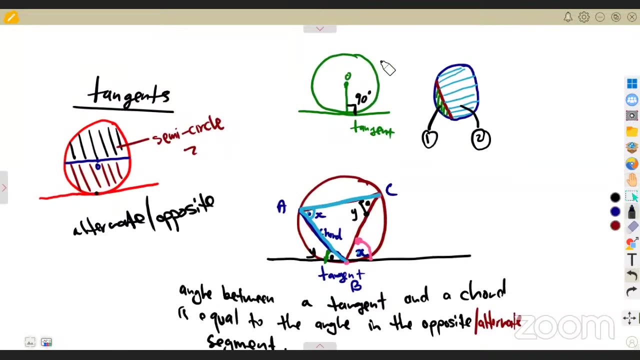 we are going to combine these theorems here, so there is a lot that it's not a lot. actually, just need to go through your theorems, understand everything. all right, so let's go back to this theorem here that I was explaining. on this part, I said: 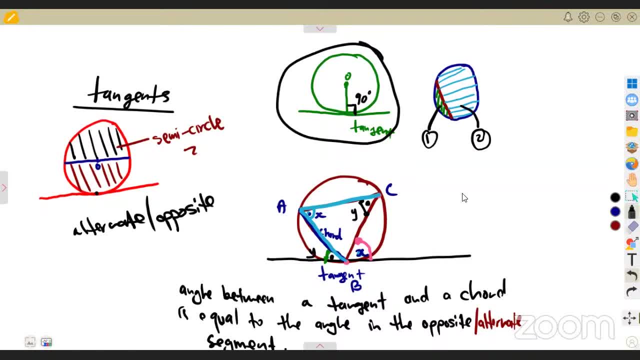 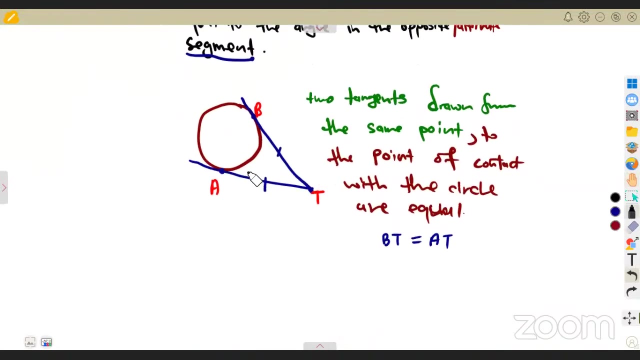 when a tangent and a radius are drawn, like where these two meet. they meet at what? at 90 degrees. now, let's bring the same here, let's bring the same here, let's say on this part that we are having here: now there was, let's say, there was- a center. 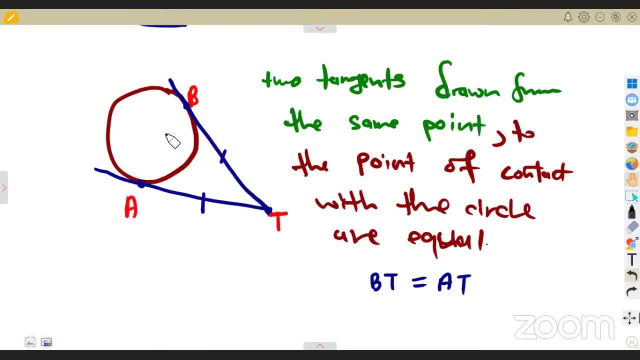 on this one, our theorem is not going to change. I'm just putting into consideration our first theorem that we had when we are dealing with tangents, the first part of our tangents. so let's say, this is our center, from O to B, that's a radius. 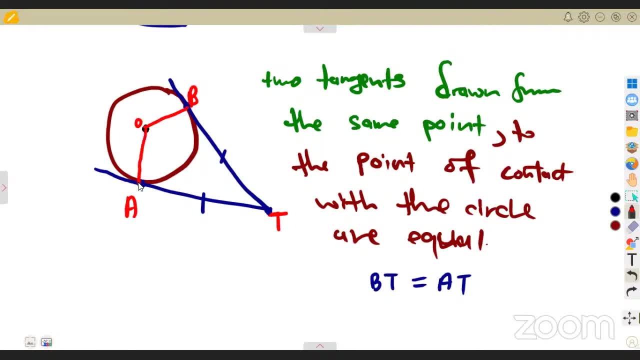 and from O to A. that's a radius. is that so? so, if this is our the case or this is the case, that O B and O A are, this is our die. so what is it that we are going to consider a radius and a tangent? we said before they meet at what? 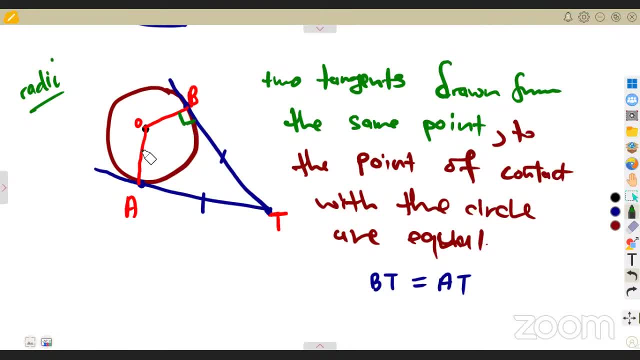 at 90 degrees a radius and a tangent. they meet at what? at 90 degrees. so it's a special type of a question that you are going to be having when it is like that, and what is it that you are supposed to consider when it is like this? 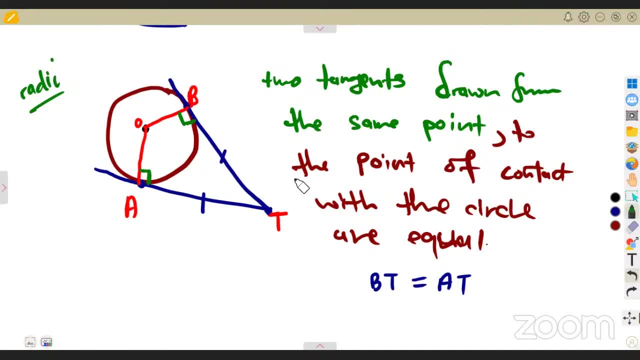 it follows that, okay, if you are referring to a quadrilateral, what is it that we know about angles in a quadrilateral? any quadrilateral, any any- a square, a rectangle, any quadrilateral, any shape with four sides? what is it that we know about the angles, angles inside? 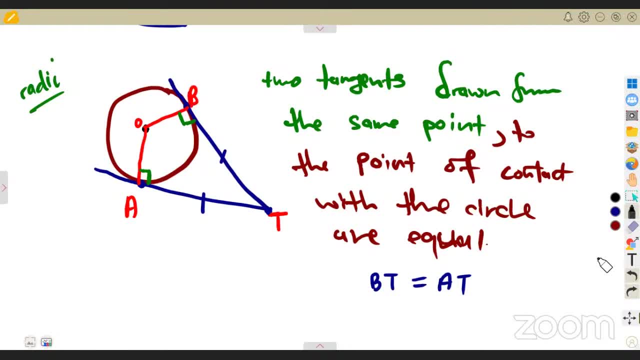 opposite angles add up to one eight. in a quadrilateral angles it's up to three sides in a quadrilateral angles is up to three sides in a quadrilateral angles is up to three sides. in a quadrilateral, all the four angles is up to 360.. 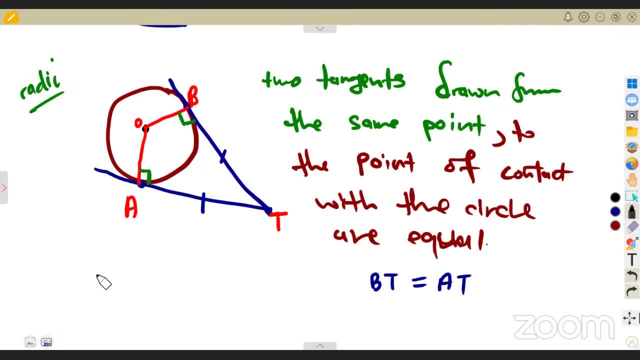 all the four angles must add up to 360.. all the four angles must add up to 360.. i'm not referring to a cyclic quadrilateral. i'm not referring to a cyclic quadrilateral. i'm not referring to a cyclic quadrilateral, no, i'm just saying a normal quadrilateral. 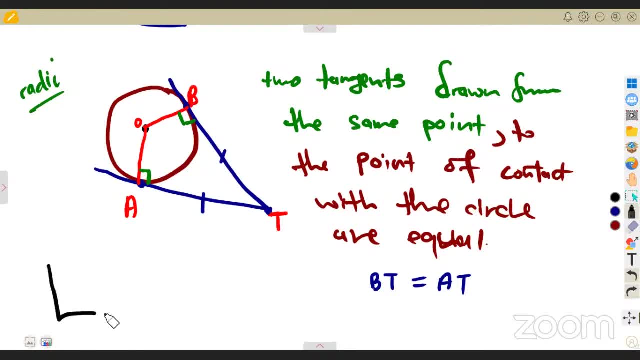 no, i'm just saying a normal quadrilateral. no, i'm just saying a normal quadrilateral. just a normal four-sided shape. just a normal four-sided shape. just a normal four-sided shape. a square, a rectangle, a trapezium as long a square, a rectangle, a trapezium as long. 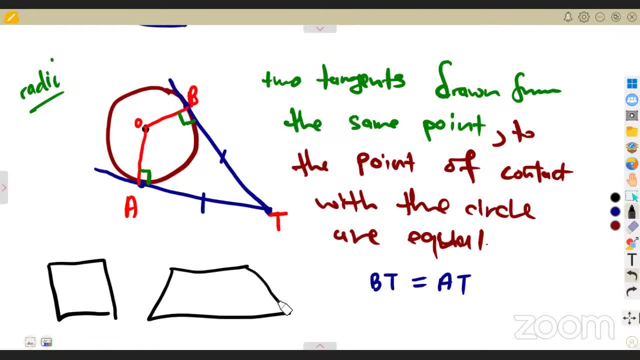 a square, a rectangle, a trapezium, as long it is. it is, it is a four-sided shape, that you are a four-sided shape, that you are a four-sided shape that you are referring to, referring to, referring to the interior angles, is 360. these are the interior angles of that quadrilateral. so if the interior angles, 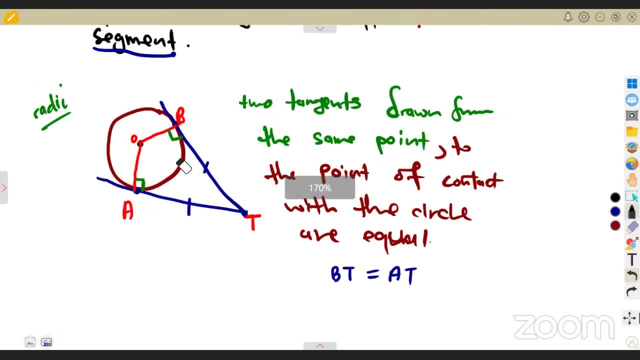 do add up to 360.. we are going to see that there is an advantage. that is happening because this angle is 90 at a. this angle at b is also 90. so 90 plus 90, it means we are now having what 180 degrees from the 90 and 90 degrees that we had from angle a and angle b. we we are now at what at? 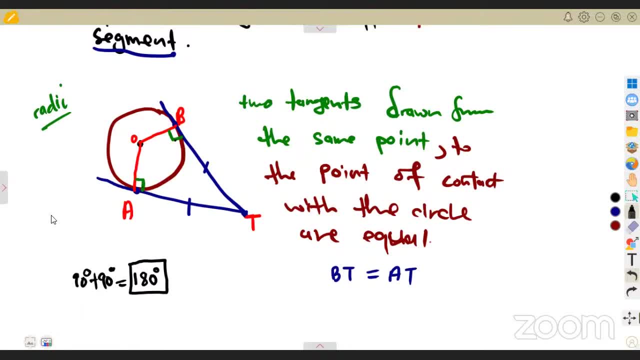 180.. so the question is: we know that every quad lateral is supposed to add up to 360 the interior angles. so if we remove this 180 that we have now, what are we going to remain with? we remain with 180.. so what does it? 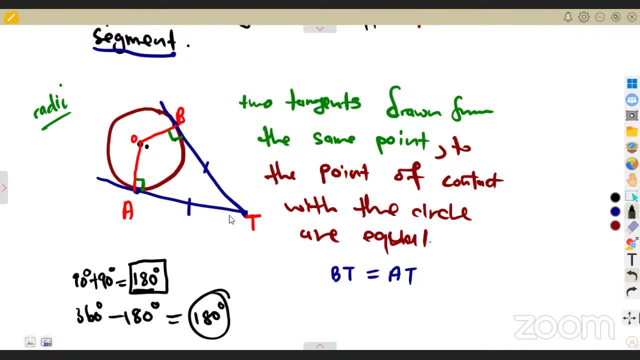 mean this angle at the center and this angle at t. they are supposed to add up to 180 degrees. so this is the special part that is only happening because of what, what happened here? the radius concept, a radius and the tangent. they meet at what? at 90.. so 90 and 90 is already gone. 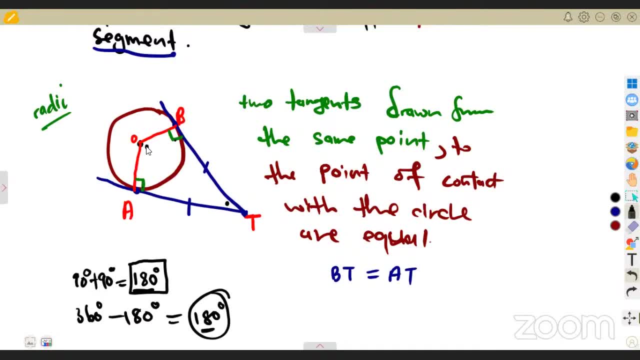 so we are remaining with 180. so therefore we can say this angle at all, which is a or b, plus the angle at t, which is you can write as a t b. all right, a t b. they must give us what 180 degrees. it's a special part that we have because of this concept. so that is something that we can. 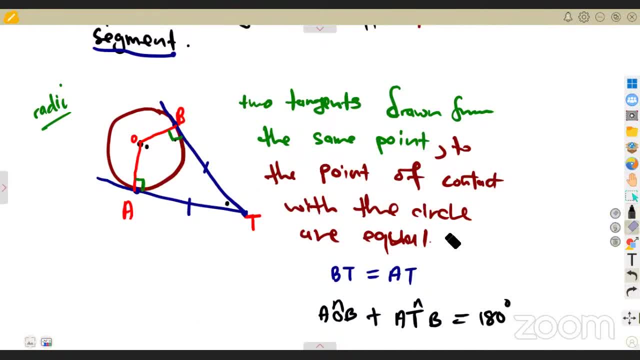 also put into consideration. also, knowing that the radius uh from or to a and from or to b is the same, these two are equal. so when the angle is at the center plus the angle at t is alsoa tb, we have 180 degrees. from o to a to b is the same, this two are equal, so we can. 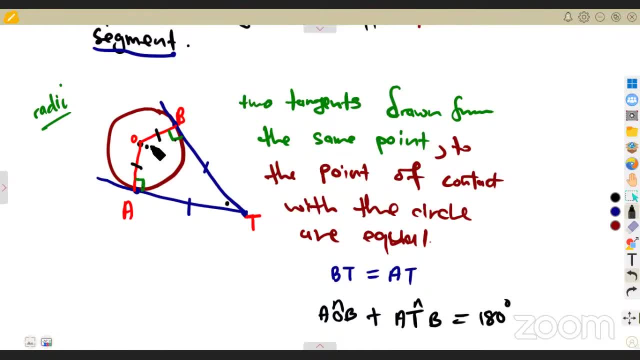 one. there's no way that we can have a radius of a circle with the three units and another radius on the same circle is four units. we are supposed to have the same length. so we can see that if we are to complete also this triangle here there's something that is happening by just completing. 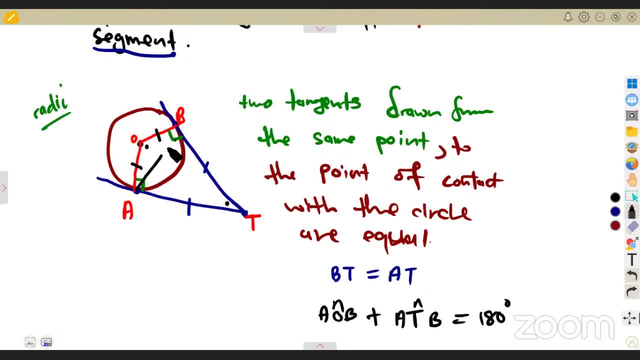 this. what is it that we can conclude? we can conclude that triangle, or a, b is what. so we are now having an isosceles triangle there, with the reason there is because of these, these two sides, which are the same. so also back to that concept: this angle and this angle will be the same. 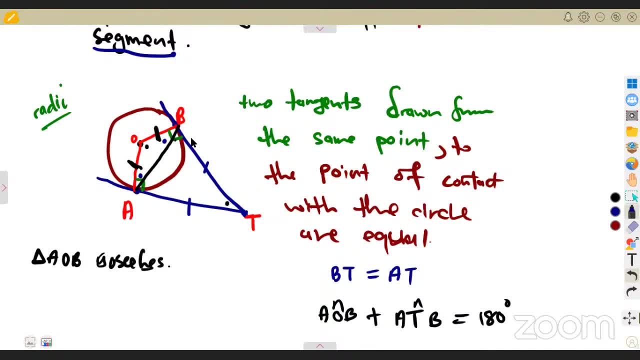 what? What about triangle, ABT, triangle, ABT, ABT, also in a source-less triangle. because of what? These two sides, which are equal. so because here I indicated these two equal, so let me just put these two here so that we see the difference. it's also in a source-less triangle. 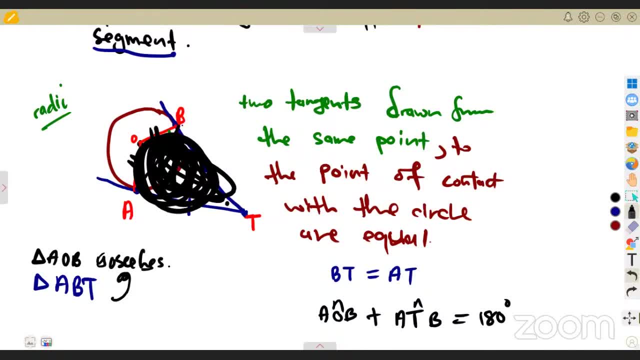 what is it that we are having now in conclusion about the whole shape like this one. now, what is what is formed? what type of a shape is that one? The kite, it's a kite. so at the end we are forming a kite. so the quadlateral formed there. 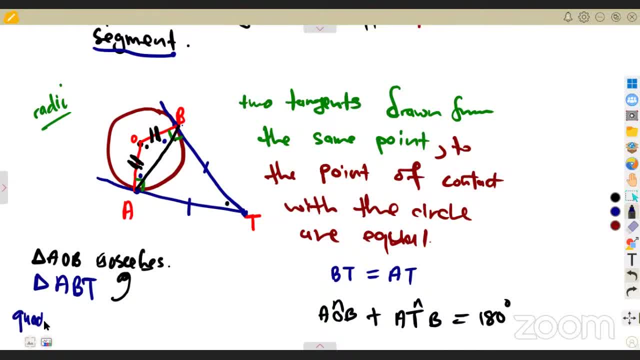 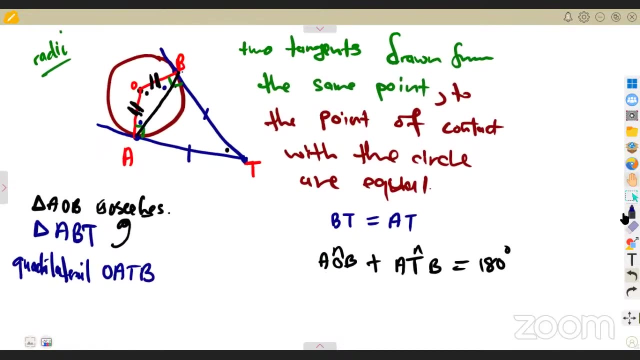 is a kite. what is the major reason that we are saying it's a kite? it's a kite, Hello. why are we saying it's a kite? because it has got pairs that are equal. so because of what these pairs of what adjacent sides equal. so whenever you have these two sides, 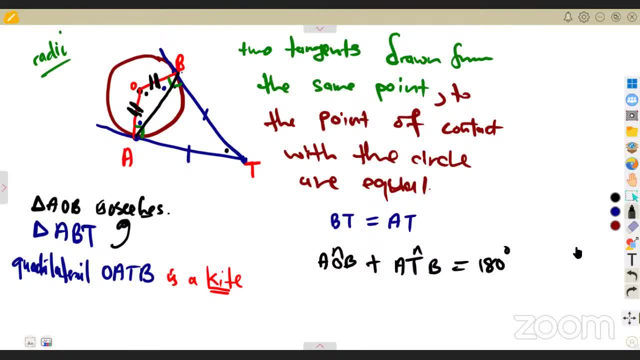 equal. these two sides equal on, Okay, Okay, What is that one? A quadlateral. that quadlateral is a kite, so it's because of what the the adjacent sides equal there's. we want to have another quadlateral like this, with these adjacent sides equal. 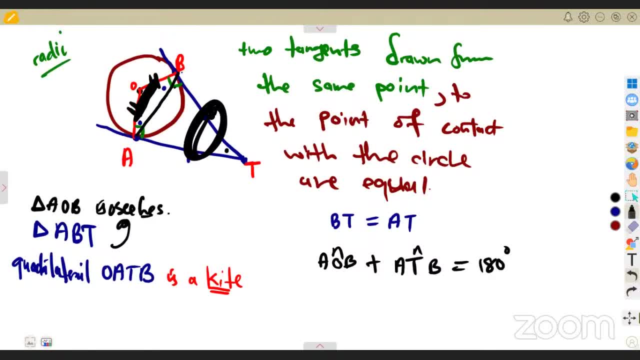 never. it's only a kite which has got these properties, so they can ask you for that special name. so we are now referring the special name, the special name of the quadrilateral o, a, t, b, depending with how you're given it, it's a what? 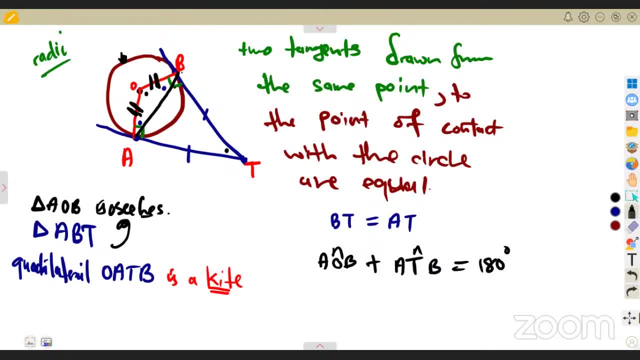 it's a kind. so these are some of the properties that you have to put into consideration. at the end of the day, all these theorems that you had on parallel, on on um, on your tangents, together combined this radius, everything now. so when you're answering questions, it's not that you're going to 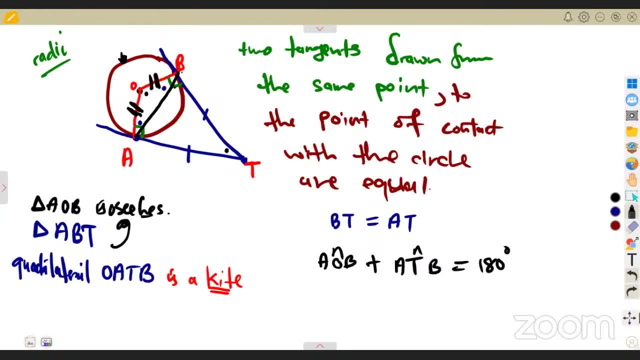 be given a something about a tangent. only you add up all theorems together, all theorems, you add up them. that is, that is how you answer now questions. every part that you have from your, from the concept, from a point, a complete revolution, angles on a straight line. all the shapes that we have. 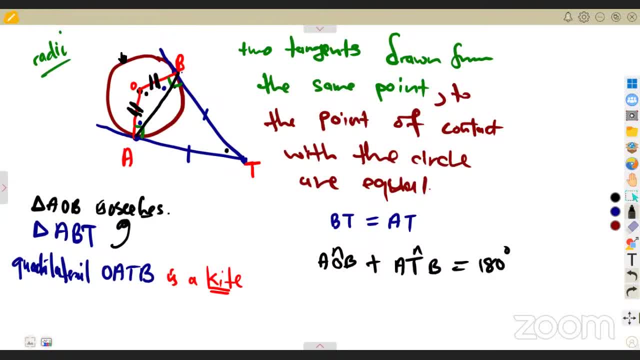 all, all, all. so, like the polygons, like that we have, we're talking of a rectangle, a square, because the moment that you're given it's a parallelogram in, maybe there's a parallelogram that you're given it has got its own properties. talk of parallel lines, all those properties. they sum up to this part of our cycle: geometry. 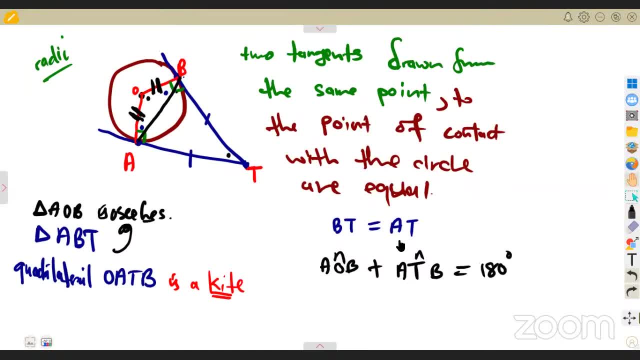 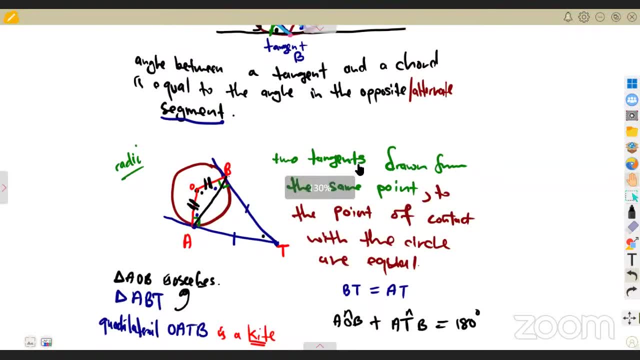 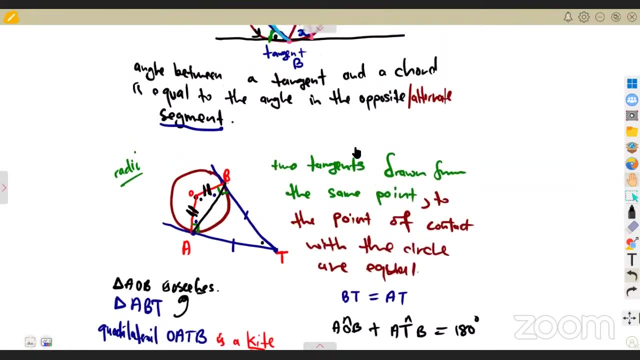 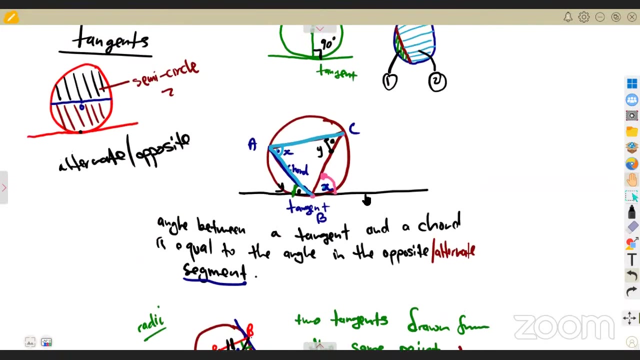 so these are the theorems that we are going to work with. uh, so i want us to add up from our previous class so that we will be able now to answer any typical exam quincent, any typical exam question. from this you can answer any typical exam question on tangents, anything that has to do with 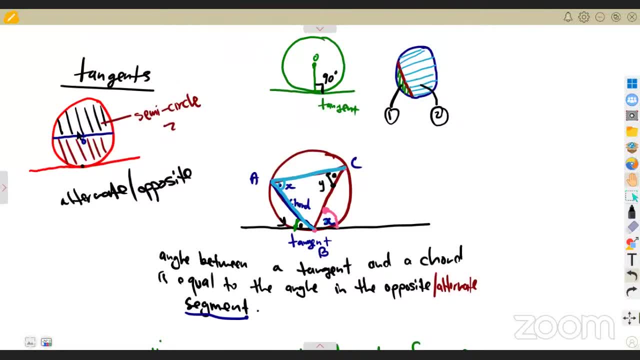 your tangents. this is what you need. so, like i Historian, i always say: let's work on with more questions. we just need to revise more question papers. the more question papers you work with, uh, the more you understand your geometry. uh, because these theorems 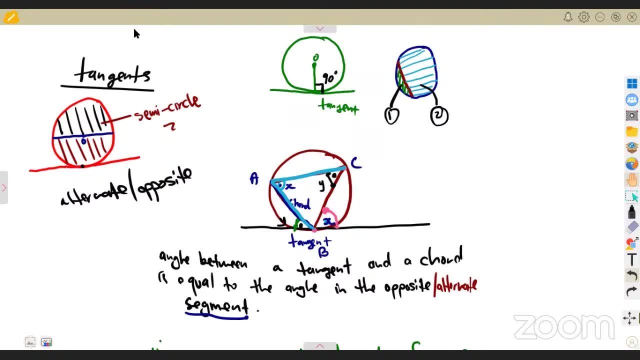 they are already. uh, they're, they're already there. you already know your theorems, so the